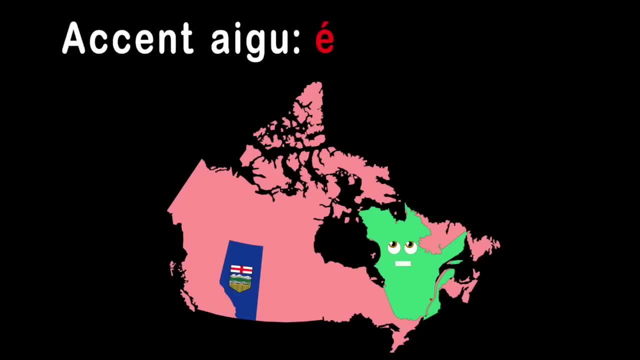 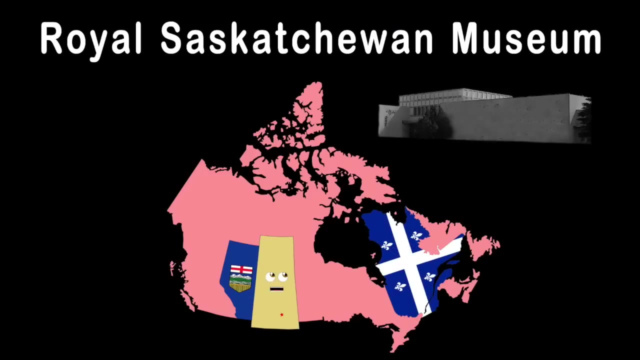 My capital is also Quebec, with an accent a-gu-e. I'm a French-speaking province of this Canadian country and I'm the largest province by area in Canada. you see, I am Saskatchewan. my capital is Regina. Royal Saskatchewan Museum is a great seat for all of ya. 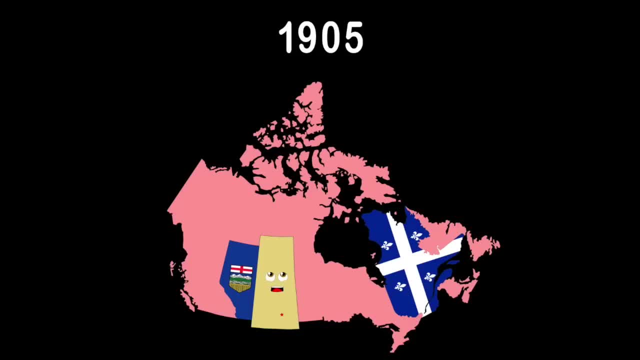 I became a province of Canada in 1905, and my provincial bird is a sharp-tailed grouse that can fly. I'm British Columbia. Victoria is my capital, Canada's westmost province, touching the Pacific coast. I have lots of mountain ranges. Whistler Mountain is my most famous. 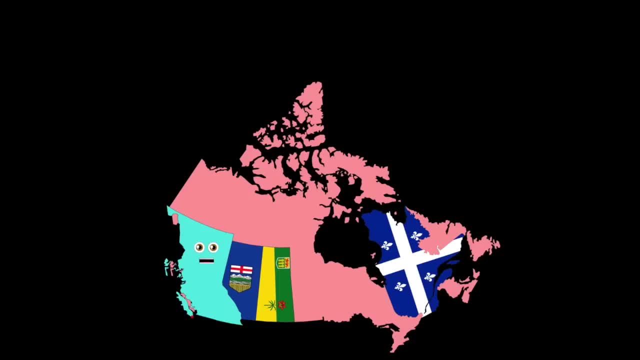 If you're looking to ski or snowboard, I have lots of these places. Hey, I'm Manitoba, My capital's Winnipeg. I'm a province of Canada. I'm not pulling your leg. Passflowers, my provincial flower. Great grey owls, my bird. 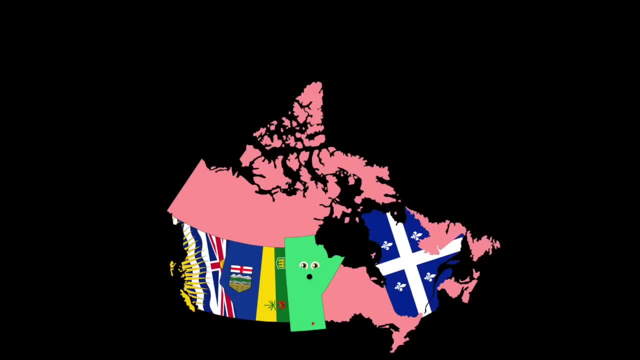 I have arctic tundra in the north and southern farmland to herd. Hey, I'm Ontario, my capital is Toronto, The Hudson Bay's to my north and the US to the south. you know, Half of Lake Ontario sits in my province, you see. 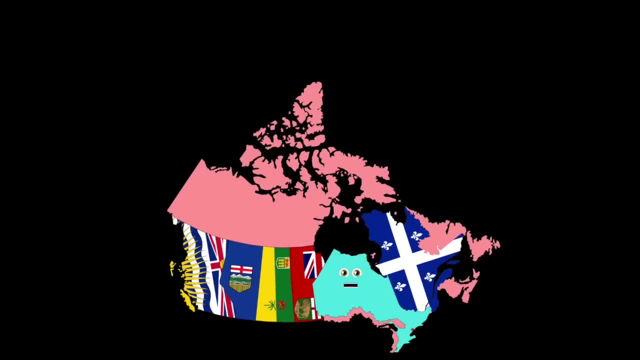 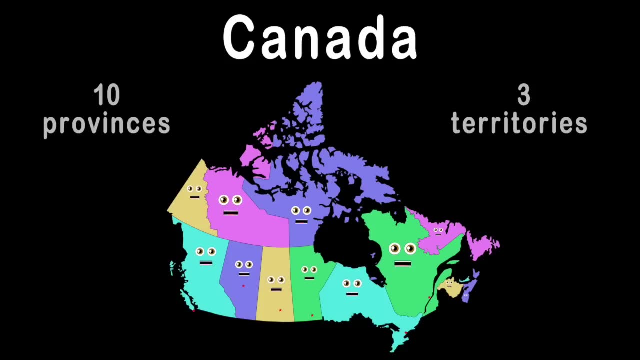 It's one of the five Great Lakes. four of them do border me. We are Canada, made up of ten provinces and three territories with capitals in all. We're here to teach you all, and then some facts that go along with them. 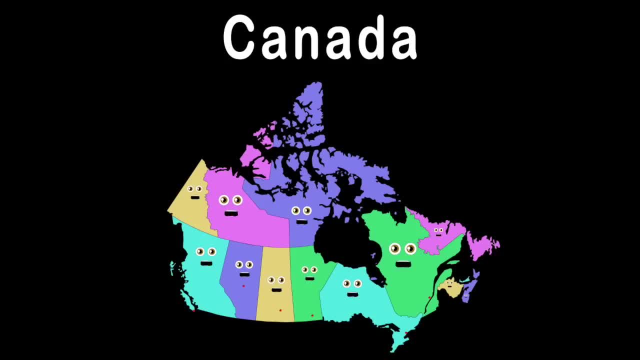 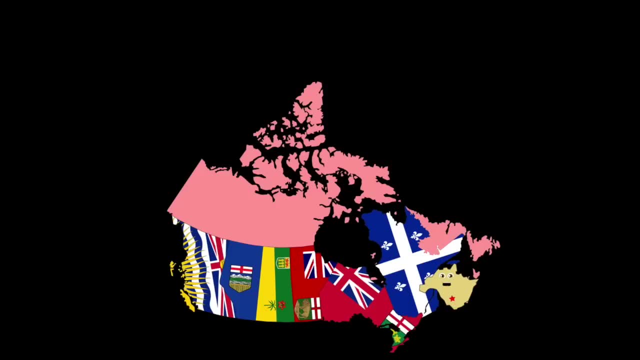 So sing along with me. now let's have a ball. Hi, I'm New Brunswick. my capital is Fredericton. I border the US state of Maine. my largest city is St John. My Bay of Fundy is most famous for its extreme tides. 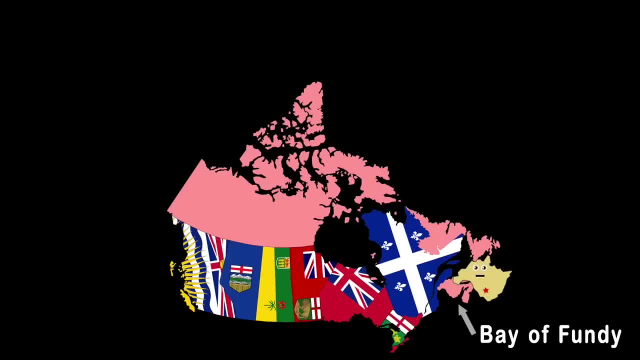 and if you're into whale watching, that's where you'd want to reside. Hello, I'm Nova Scotia. my capital's Halifax. I'm one of Canada's maritime provinces. now, how about that? I'm in the Atlantic Ocean. I also have long coastlines. 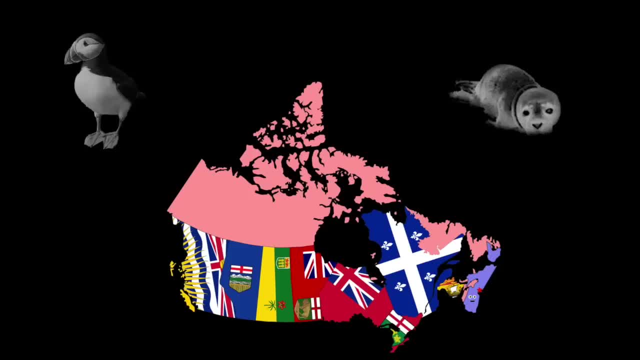 I'm home to the puffin and seals. yeah, my scenery is fine. I'm Prince Edward Island. my capital is Charlottetown. I'm a Canadian province and, where the province house is found, I am known for my seafood.